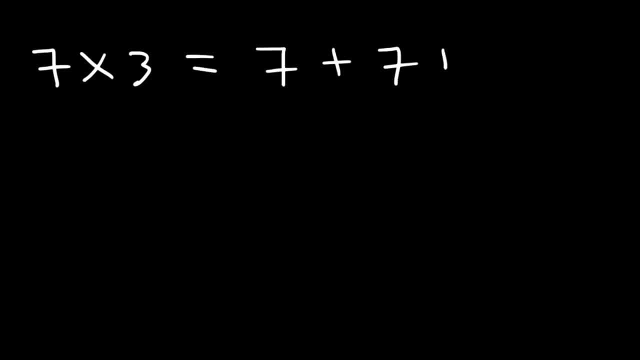 It's equivalent to adding 7 three times. 7 plus 7 is 14.. 14 plus the other, 7 is 21.. Therefore, 7 times 3 is 21.. And so multiplication is simply just addition multiple times. 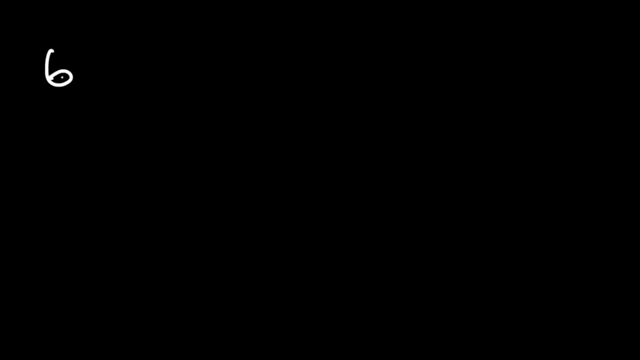 So now let's work on some examples. What is 6 times 5, and what is 4 times 8?? Feel free to pause the video and work on these two examples. 6 times 5 is equivalent to adding 6 five times. 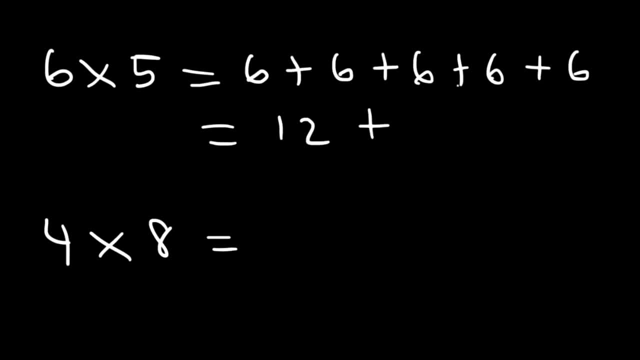 6 plus 6 is 12.. So the other two 6s will add up to 12, and we have one 6 left over. 12 plus 12 is 24.. 24 plus 6 is 30. And so that's the answer for the first one. 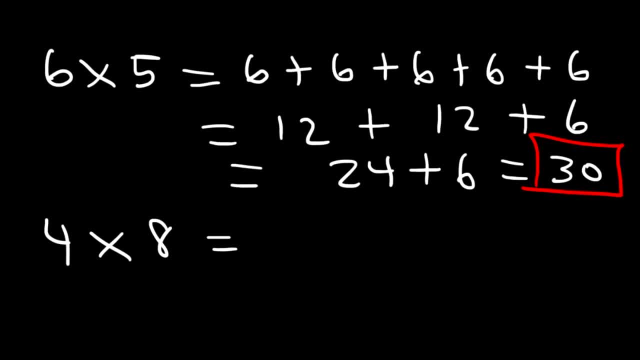 Now 4 times 8. We can add 4 eight times or add 8 four times. Let's add 8 four times, since it involves less writing. 8 plus 8 is 16.. And so the other two 8s add up to 16.. 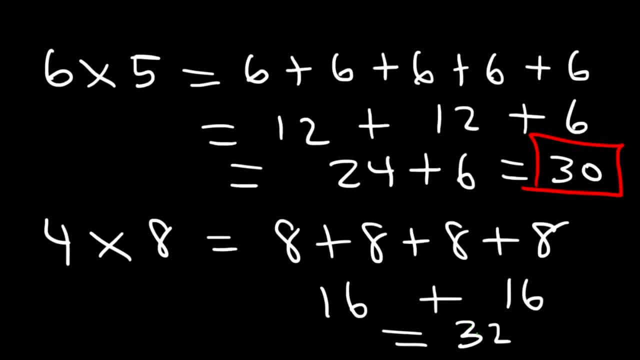 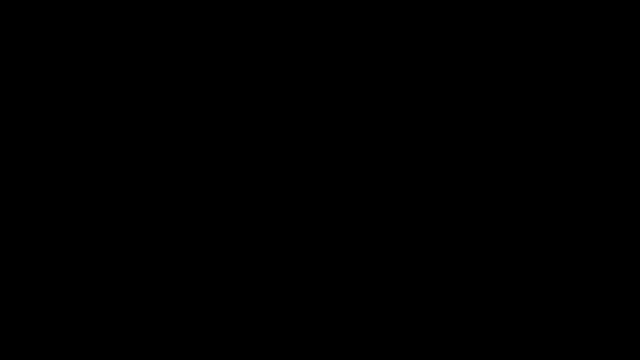 16 plus 16 is 32.. Therefore, 4 times 8 is 32.. Now, what exactly is division? Division is the opposite of multiplication. For instance, we know that 4 times 5 is equal to 20.. Therefore, 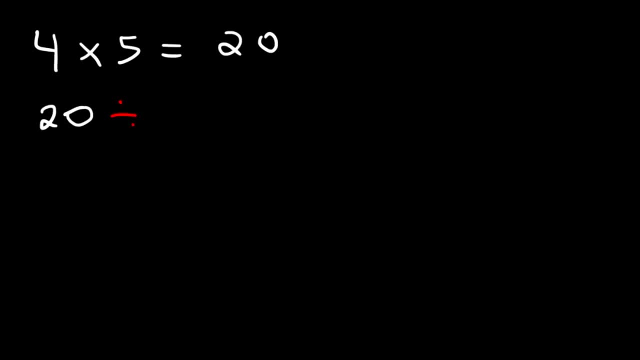 20 divided by 5 is equal to 4.. You can also say that 20 divided by 4 is equal to 5.. And so if you know how to multiply, you know how to divide. Division is simply the opposite of multiplication. 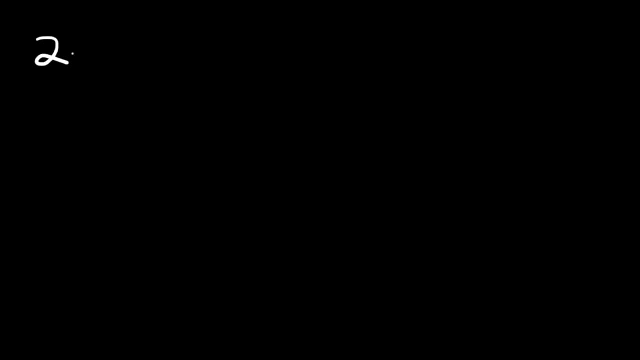 So, with that in mind, what is 28 divided by 4?? So ask yourself 4 times, what number is 28?? How many times do I have to add 4 to get to 28?? You have to add it 7 times. 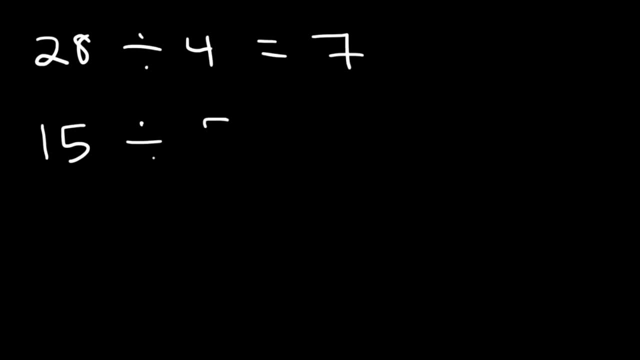 Here's another example: What's 15 divided by 5? 5 times, what number is equal to 15?? How many times do I have to add 5 to itself to get to 15?? 5 plus 5 is 10.. 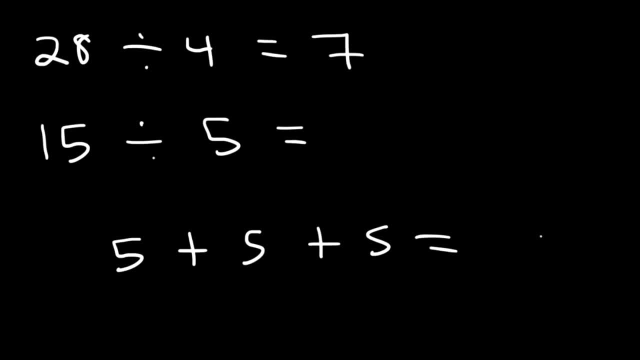 10 plus 5 is 15.. So I need to add 3- 5s to get to 15.. Therefore, 15 divided by 5 is 3.. Let's work on a few more examples. So what is 12 divided by 5?? 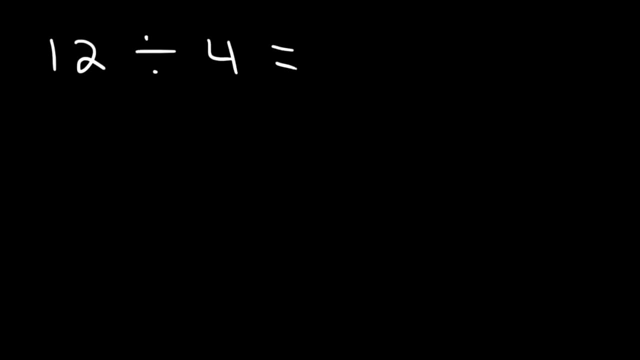 So what is 12 divided by 5?? 4 divided by 4. Or 4 times, what number is equal to 12?? How many times do I have to add 4 to get to 12? 4 plus 4 is 8.. 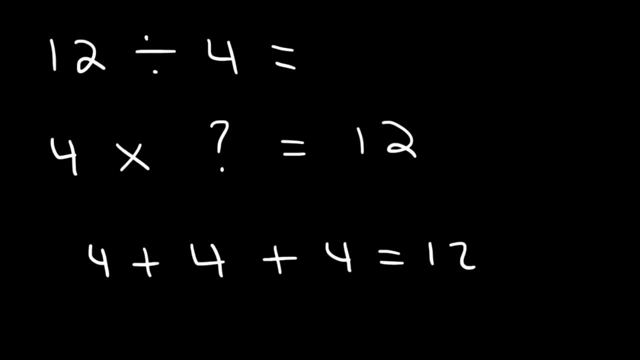 8 plus 4 is 12.. So I have to add 3- 4s to get to 12.. Therefore, 4 times 3 is 12. And 12 divided by 4 is 3.. And so this is the answer. 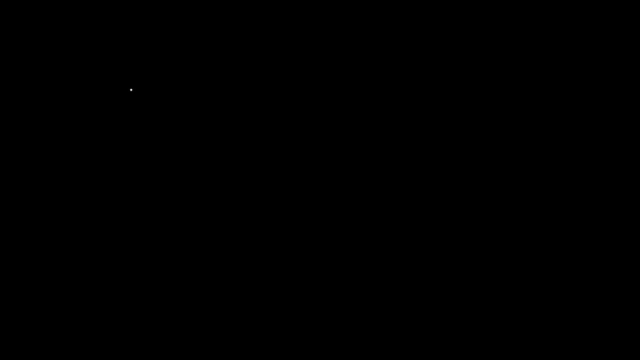 And so that's the answer. Now, what is 36 divided by 9?? Now, what is 36 divided by 9?? So 9 times what number is 36?? So 9 times what number is 36?? How many times do I have to add 9 to get to 36?? 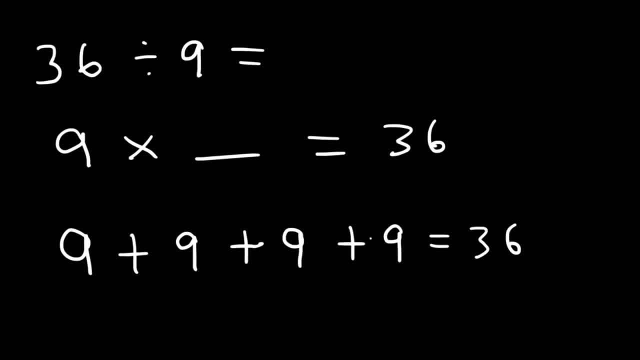 is 27, 27 plus 9 is 36.. So you have to add 9 four times to get to 36.. Thus, 9 times 4 is 36, and 36 divided by 9 is 4.. So now you see the relationship between multiplication and division. 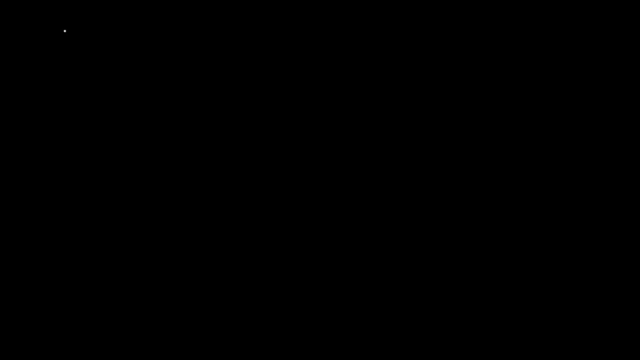 Now let's talk about multiplying two large numbers. What is 20 times 13?? Now think about it: If you have 13 $20 bills, how much money do you have? Well, we know that 5 $20 bills adds up to 100, which means 10 $20 bills add up to 200, and 3: 20s is 60. 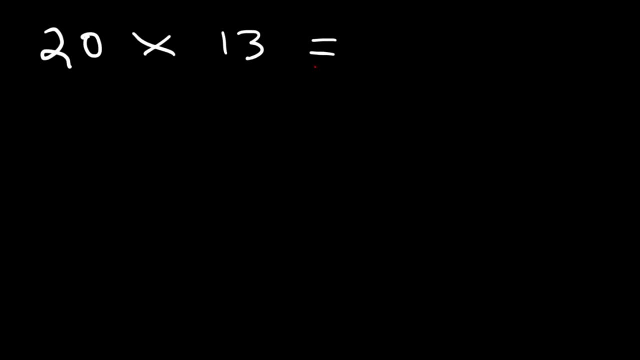 So the total is $260.. So 20 times 13 is 260.. Whenever you can conceptualize numbers and apply it to something that you can visualize, it becomes easier to understand. Most people understand how to count money, And so if you can relate numbers to money, it's going to be easier to do multiplication. 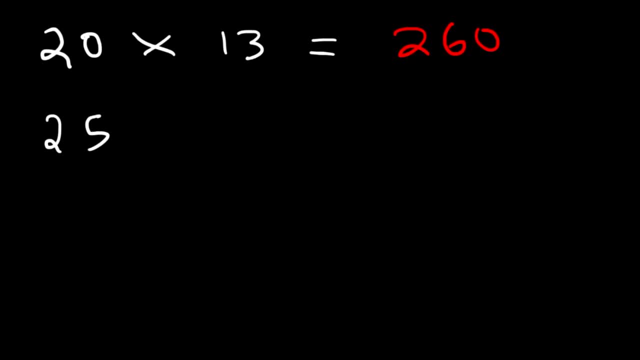 Here's another example. Let's say if we want to multiply 25 by 15.. Ask yourself what is the value of 15 quarters. You know, 4 quarters add up to $1.. 8 quarters is $2.. 12 quarters add up to $3.. 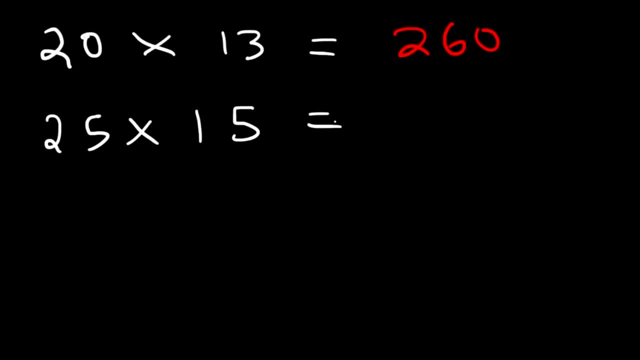 And we want to get up to 15 quarters. so the other 3 quarters is $0.75.. 15 quarters is $375.. Therefore, 25 times 15 is $375.. So if you can visualize numbers, it can help you to do math. 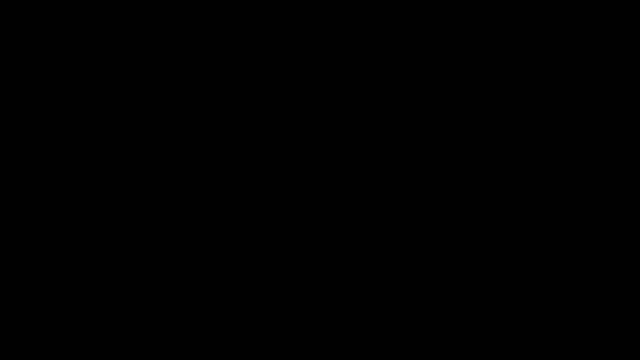 But let's say, if you want to calculate it by hand, You can also do it this way. So first you want to multiply 5 times 5.. 5 times 5 is 25.. Carry over the 2.. 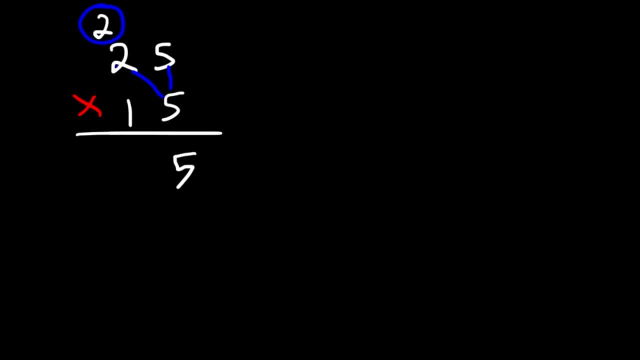 And then 5 times 2 is 10 plus 2.. That's going to be 12.. Next add a 0.. 1 times 5 is 5.. 1 times 5 is 5.. And 1 times 2 is 2.. 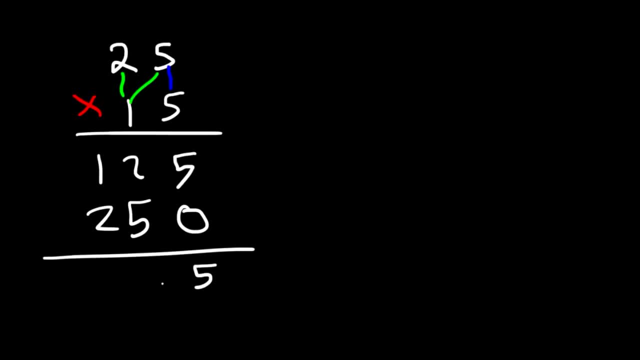 And now let's add: 5 plus 0 is 5.. 2 plus 5 is 7.. 1 plus 2 is 3.. And so you get 375.. So that's how you can multiply by hand if you don't have access to a calculator. 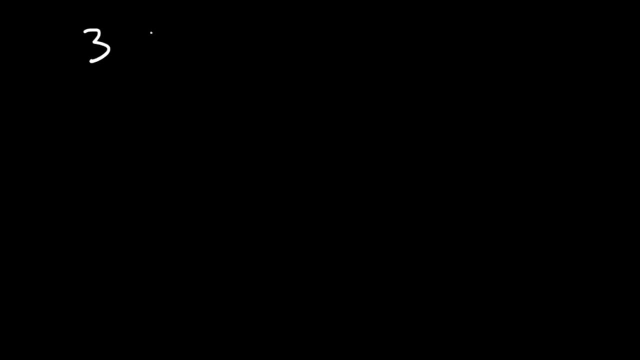 Let's try another example for the sake of practice. So go ahead and multiply 36 by 42.. Feel free to pause the video. 2 times 6 is 12.. Let's carry over the 1.. And then 3 times 2 is 6 plus 1.. 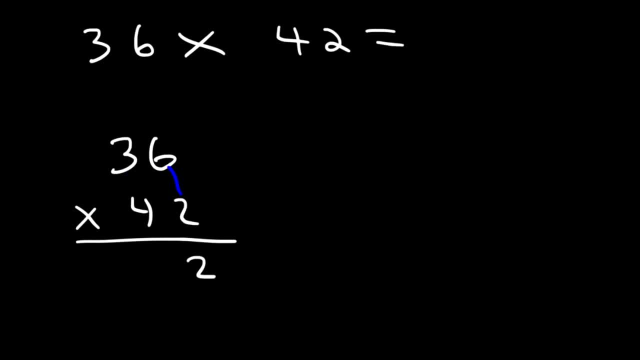 That's 7.. Now we need to add a 0.. 4 times 6 is 24.. Let's write the 4. Carry over the 2. And then 4 times 3 is 12, plus 2, that's going to be 14.. 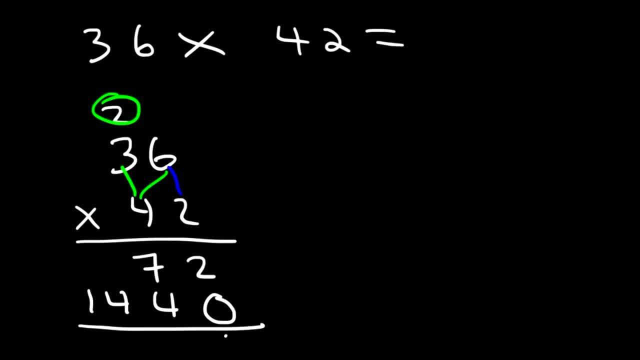 So now let's add: 0 plus 2 is 2,, 4 plus 7 is 11,. carry over the 1,, 4 plus 1 is 5, and bring down the 1.. So 36 times 42 is 1512.. 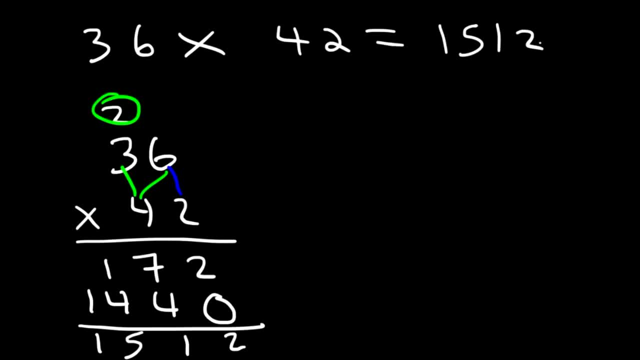 And you can type it in the calculator to confirm that answer. So that's how you can multiply two large numbers. Now let's talk about division. What if we wanted to divide a large number by a small number, like 3?? Now you don't want to keep adding 3 until you get to 105. 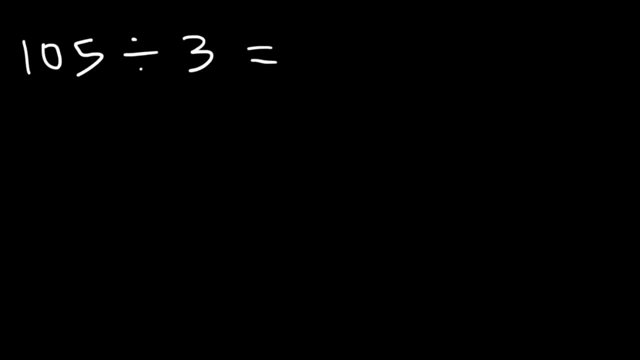 That's going to take a long time, So instead you want to use a process called long division. Long division will help you to figure out what exactly 105 divided by 3 is. Let's put the 3 on the outside And 105 on the inside. 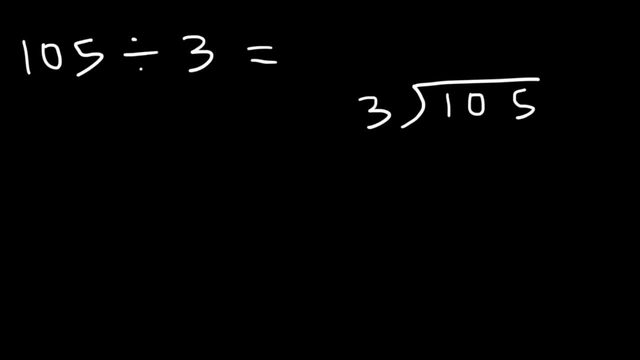 3 doesn't go into 1, because 3 is less than 1.. However, 3 can go into 10.. How many times does 3 go into 10?? 3 times 3 is 9.. 3 times 4 is 12,, which is too much. 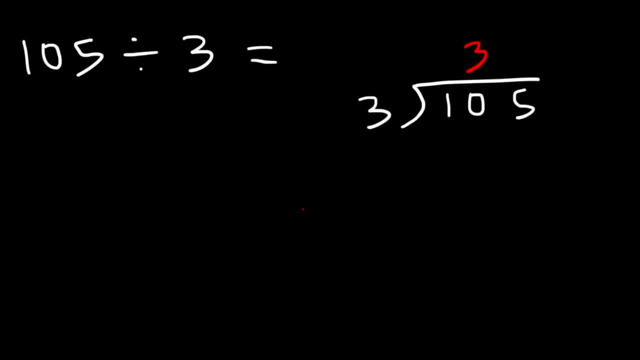 So 3 can go into 10 three times, since 3 times 3 is 9.. And now let's subtract: 10 minus 9 is 1. And let's bring down to 5.. How many times does 3 go into 15?? 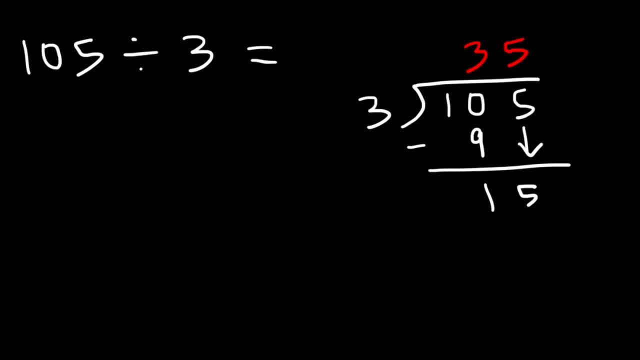 3 goes into 15. five times 3 times 5 is 15. And the remainder is 0. So 105 divided by 3 is equal to 35.. Now let's try another example. What is 184 divided by 4?? 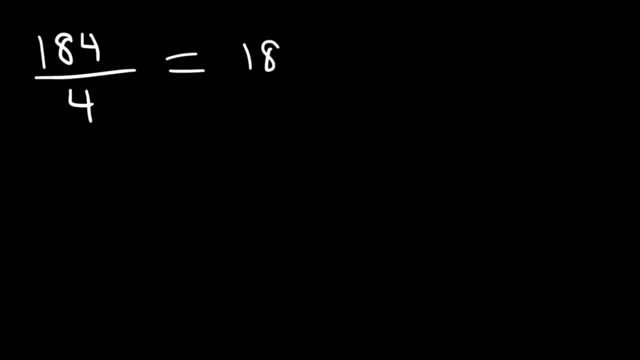 If you see it written as a fraction, it's equivalent to this expression. So let's divide these two numbers. How many times does 4 go into 18?? 4 goes into 18 four times. 4 times 4 is 16.. 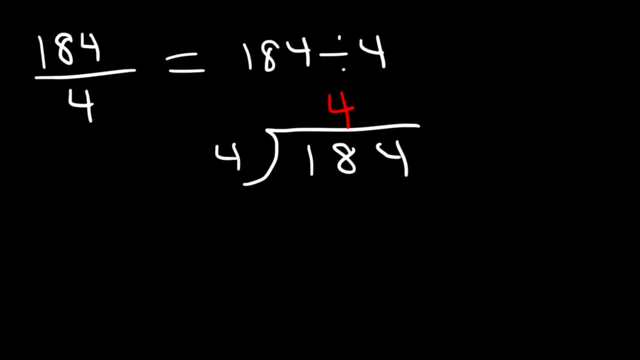 And 18 minus 16 is 2.. Now let's bring down to 4.. 4 goes into 24 six times. 4 times 6 is 24.. And the remainder is 0. So therefore, 4 goes into 24 six times.